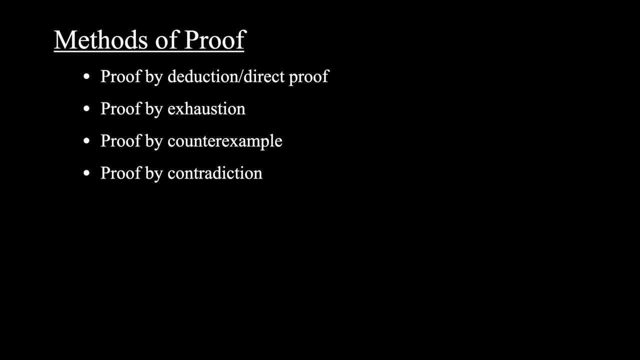 by deduction, also known as direct proof, proof by exhaustion, proof by counterexample and proof by contradiction. There is also some terminology you should be aware of. Firstly, a statement is the thing you're trying to prove, So typically a proof question will start with a statement. 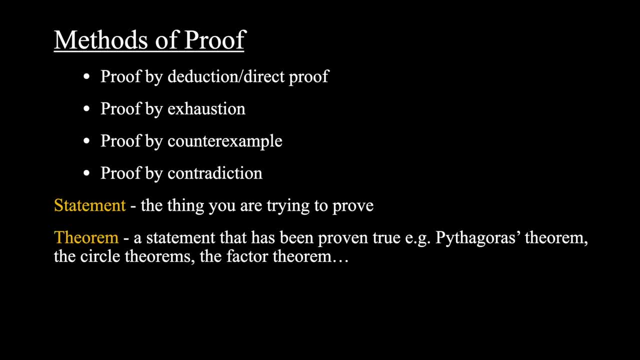 that is either true or false. You need to go ahead and prove that A theorem is a statement that has been proven true. For example, Pythagoras's theorem, the circle theorems, the factor theorem, the list goes on and on, And actually, if you want to see a list of the hundred greatest theorems of 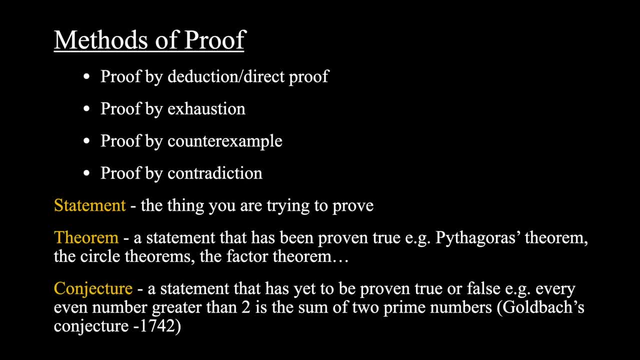 all time. I'll leave a link in the description, And a conjecture is a statement that has yet to be proven true or false. For example, every even number greater than two is the sum of two prime numbers. This is a famous conjecture, known as Goldbach's conjecture Originally. 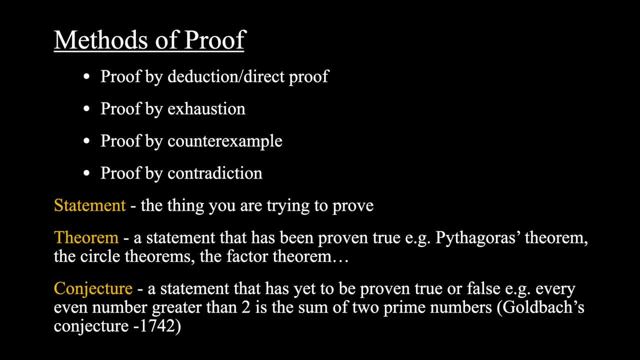 stated in 1742 and yet to be proven true or false. So before we prove a statement, we can refer to it as a conjecture. Once we prove it, we can call it a theorem. And, by the way, if you prove this conjecture, you will get one million dollars. So there you go, if you want to make one million. 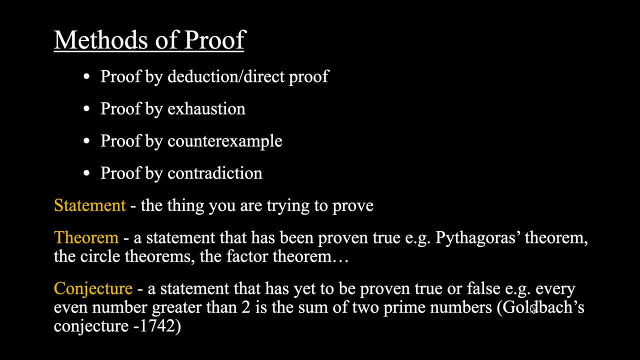 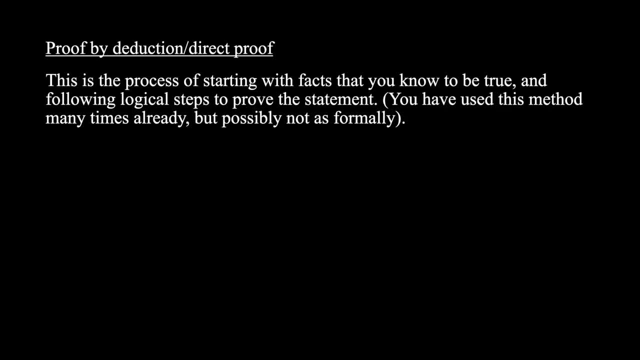 dollars, just go ahead and prove Goldbach's conjecture. Okay, on to the first method of proof. This is proof by deduction, also known as direct proof. This is the process of starting with facts you know to be true and following logical steps to prove the statement. I would say: 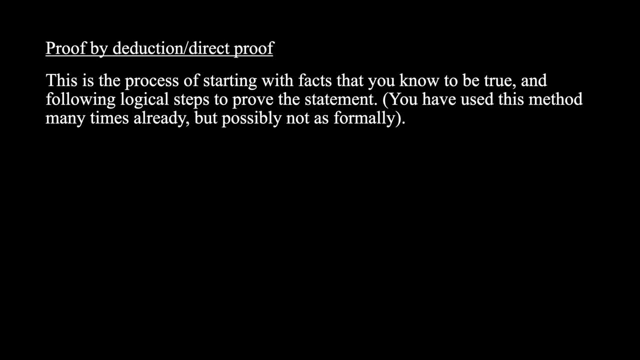 this is the most straightforward method and one that you have used many times already. Think of all of those circle theorem problems that you solved in GCSEs and the vector proof questions. They were methods of proof by deduction, So let's look at an example. Firstly, we start with the 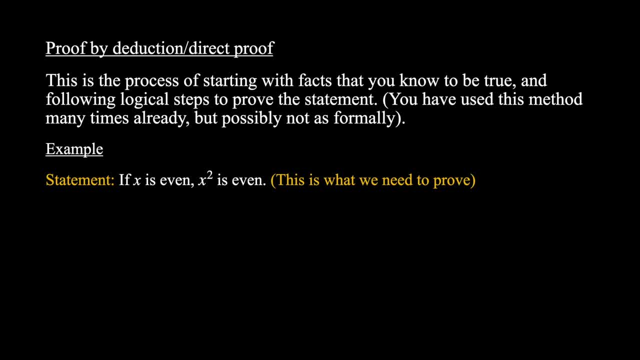 statement. This is what we need to prove. This statement says: if x is even, x squared is even. And to use proof by deduction, you want to start with a known fact, something that you know is true. So here we're going to start with the fact that if x is even, 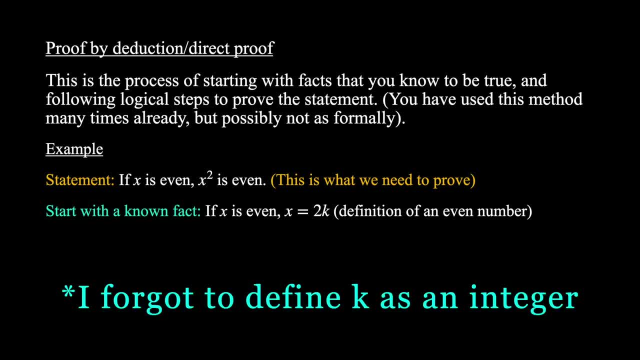 If x is even, x squared is equal to 2k. This is the definition of an even number. Every even number is a multiple of 2.. That's what we're saying here. with x equals 2k, Then the next logical step is to square x, So x squared equals 2k squared, which is 4k squared, and we can factorize. 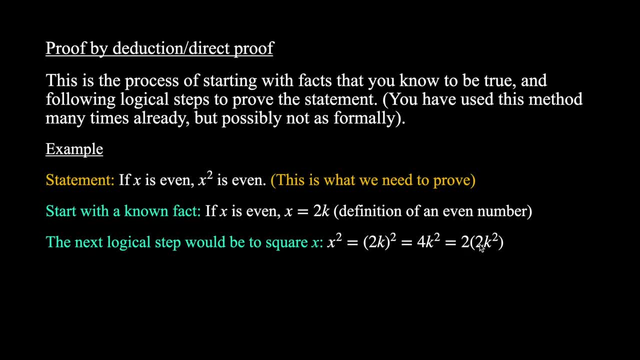 the 2 out and then write it as a multiple of 2.. So x squared is 2 multiplied by 2k squared. Then we can see that this is a multiple of 2, and a multiple of 2 is, by definition, an even number. 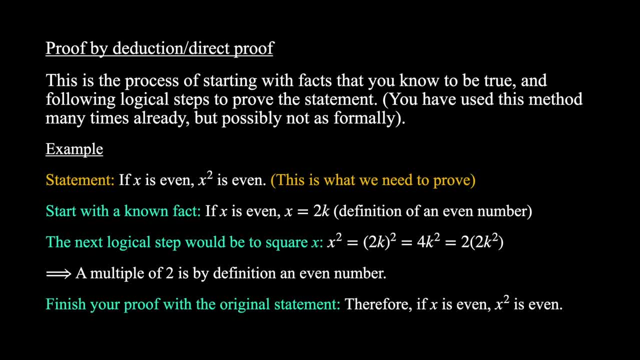 So we want to finish your proof off with the original statement. So we can say, therefore, if x is even, x squared is even. So that's an example of proof by deduction. You start with some known fact that you know to be true and you follow some logical steps to prove the original. 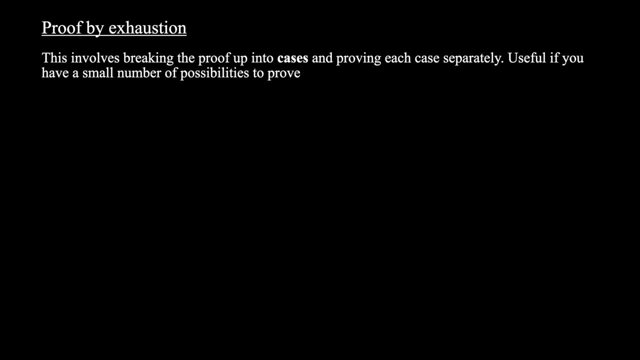 statement. On to the next one, proof by exhaustion. This involves breaking the proof up into cases and proving each case separately. This is useful if you have a small number of possibilities to prove. So let's look at an example. So we're going to create aריable and a multiple of 4.. So we're going to make a multiple of three. 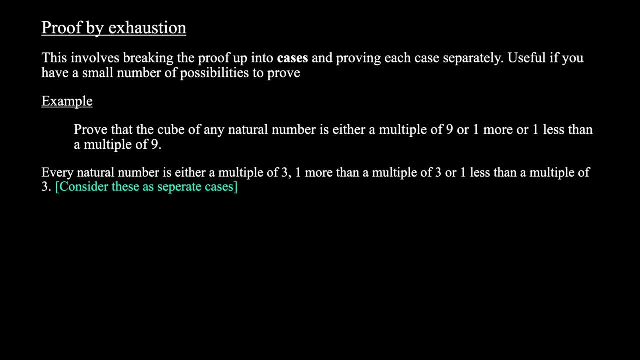 or one less, and then we're going to consider these as separate cases. So for multiples of three, if we cube those, that would be 3k cubed, which is 27 k cubed, and we can factor a nine out and we'd get nine multiplied by 3k cubed. This is a multiple of nine. In the next case we're going to write: 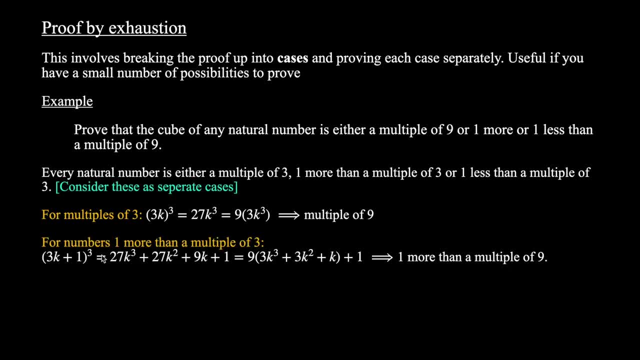 We can consider the numbers one more than a multiple of three. so we can represent that as 3k plus one and we cube that. we would get 27k cubed plus 27k squared plus 9k plus one. Now I skipped some steps there. 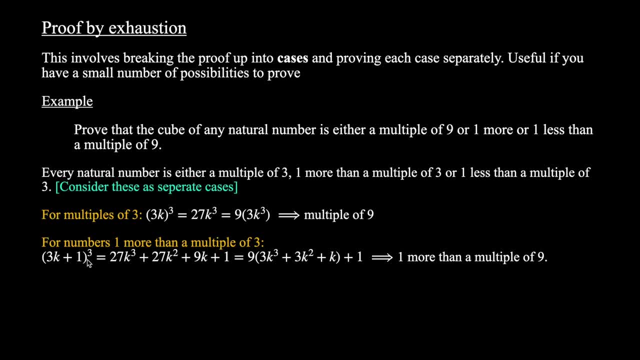 We could either use a binomial theorem to expand those brackets or expand them out the long way. so multiplying the first set of brackets and then multiplying a quadratic by 3k plus one Once you expand the brackets out, this is what you get. 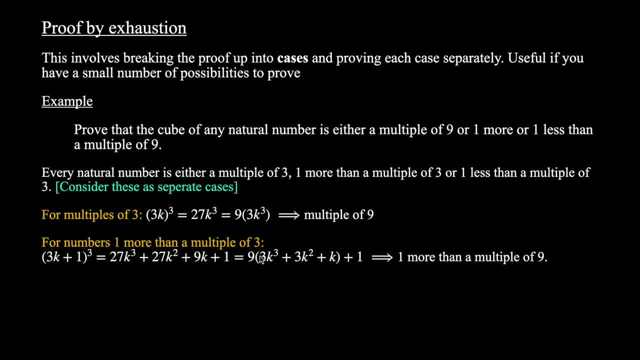 Then we can factorize a nine out of the first three terms and then we get nine multiplied by 3k cubed, plus 3k squared plus k, and then we have that plus one on the end. So this is clearly a multiple of nine plus one. so this is one more than a multiple of 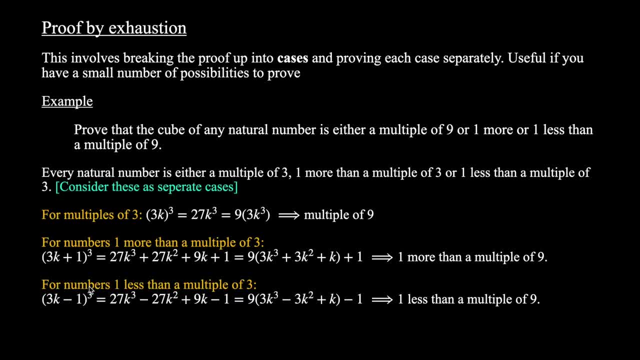 nine. Then the last case we need to consider is numbers less than a multiple of three. This would be 3k. take one cubed. Expanding this out as we did for the second case, we would get 27k cubed plus 3k squared. 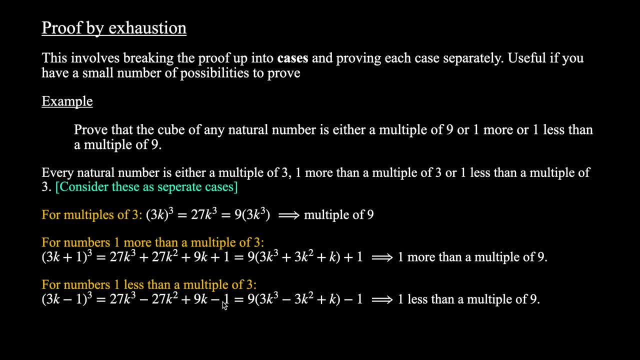 plus 9k. take one. factorizing nine out of the first three terms, we get nine multiplied by 3k. cubed. take 3k. squared plus k, take one. This is one less than a multiple of nine. and now we have actually considered all possible. 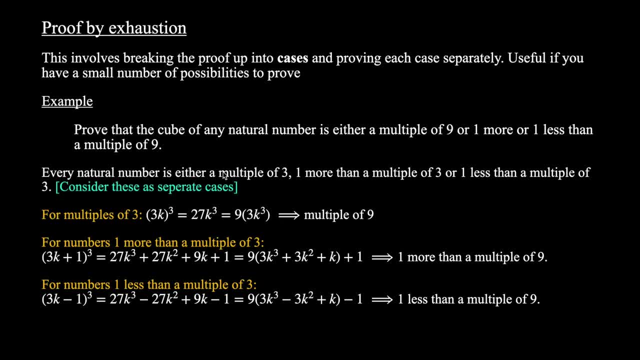 natural numbers because, as we said at the start, every natural number is either a multiple of three, one more than one less than a multiple of three. So we've considered all natural numbers in these three cases and we can conclude the proof with the statement. 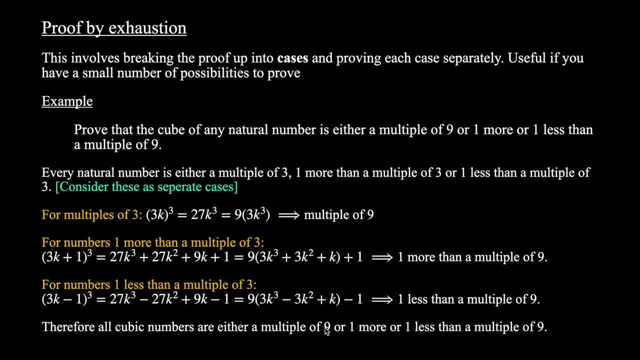 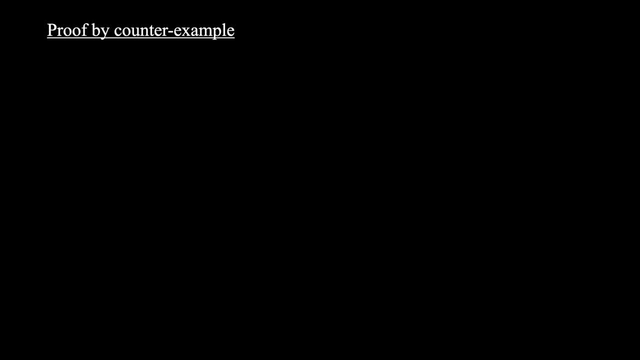 So we can say: Therefore, all cubic numbers are either a multiple of nine, one more than, or one less than a multiple of nine. So that is proof by exhaustion. The next one, proof by counterexample. This is where you prove that the statement is false by giving an example that shows the 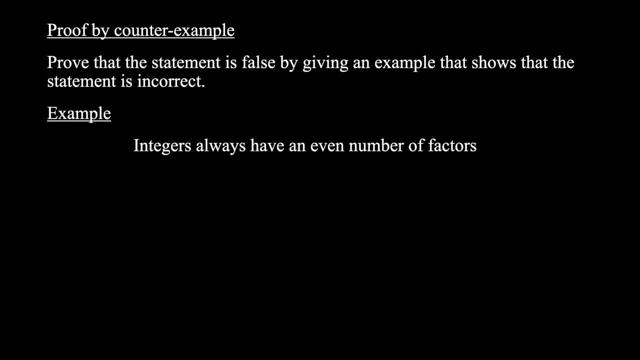 statement is incorrect. So let's look at an example Here. the statement says integers always have an even number of factors. What we want to do is try to think of a counterexample that shows this is not true, So the most obvious one I could think of was one. 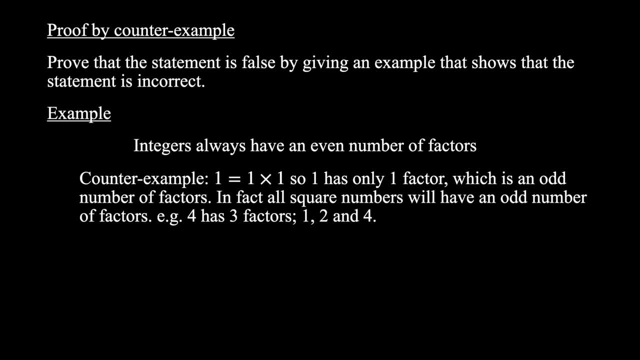 Because one equals one times one. they're the only factors of one. So one has only one factor, which is an odd number of factors, And in fact all square numbers will have an odd number of factors. For example, four has three factors: one, two and four. 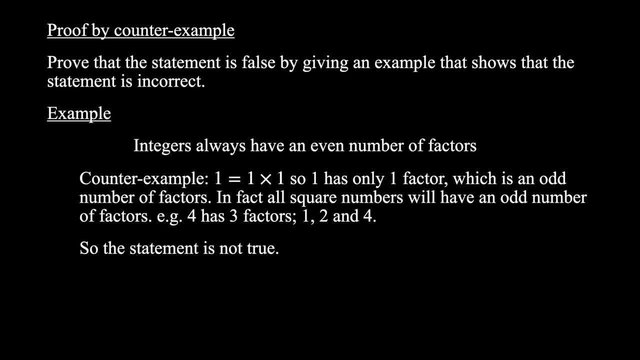 So because we provide that counterexample, we can say the statement is not true. A fairly well-known historical example involves the mathematician Fermat. In the 1600s he conjectured that two to the power of two to the power of three is not. 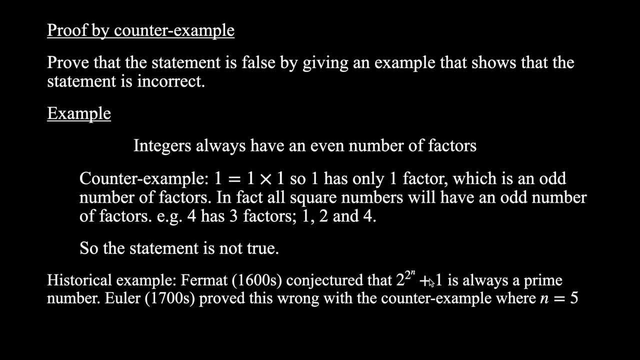 true, So we can say the statement is not true. So we can see that the number of factors always has an even number of factors, which is a prime number. And Euler, another mathematician in the 1700s, proved this wrong with the counterexample. 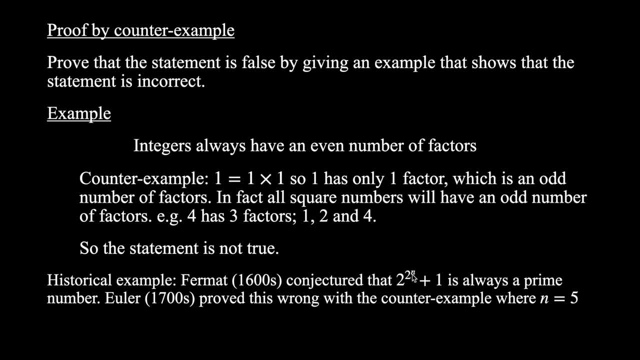 where n equals five. So it seems like Fermat tried n equals one, two, three and four, and then maybe he couldn't be bothered working out when n equals five. So he just said it's always a prime number. But you can probably forgive him, considering that two to the power, of two to the power. 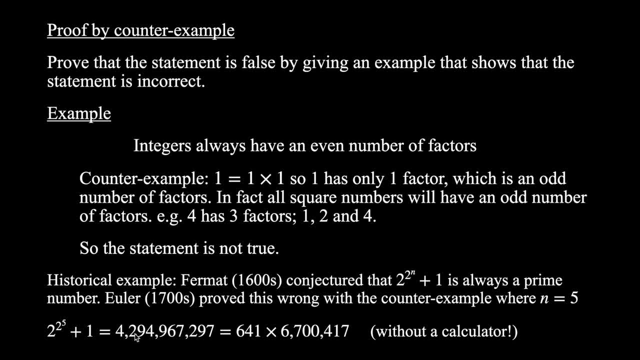 of five plus one is 4,21,000,000.. So he can probably forgive him just for that. He can probably forgive him for that 294,967,297, which equals 641 multiplied by 6,700,417.. And Euler figured this out without. 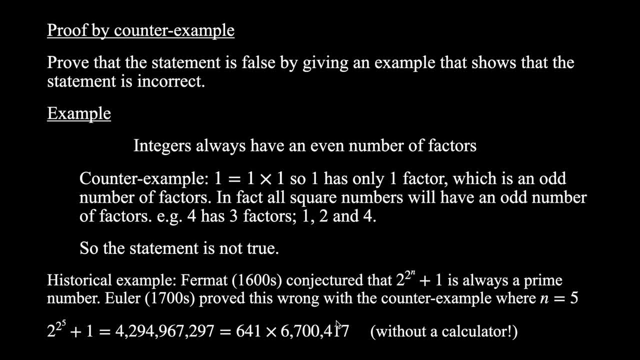 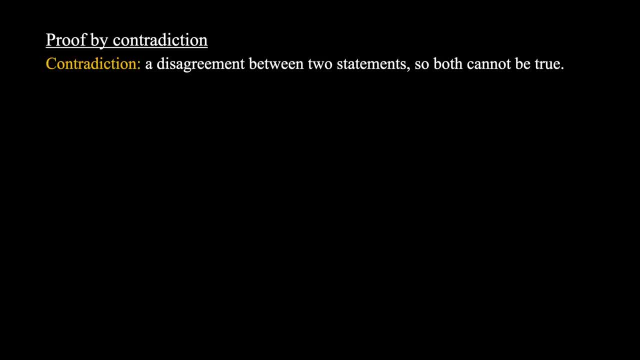 a calculator. Pretty impressive stuff. So there's a famous example of proof by counter example. The last one we're going to look at is proof by contradiction. Firstly, what is a contradiction? A contradiction is a disagreement between two statements, So both cannot be true, For example, 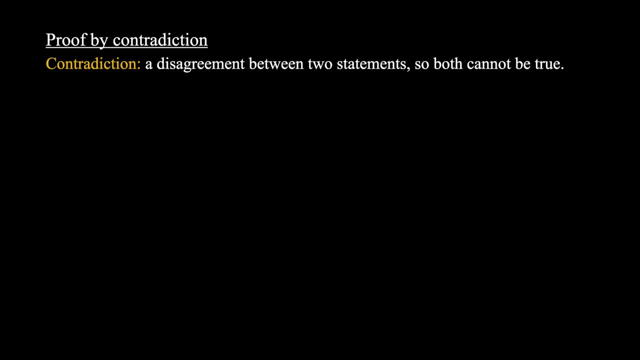 I could say something ridiculous to my mother. like mom, when you're my age, you'll understand. That's a contradiction, because clearly, if she's my mom, she's older than me, right? So implying that she's younger than me is a contradiction. Proof by contradiction then involves assuming: 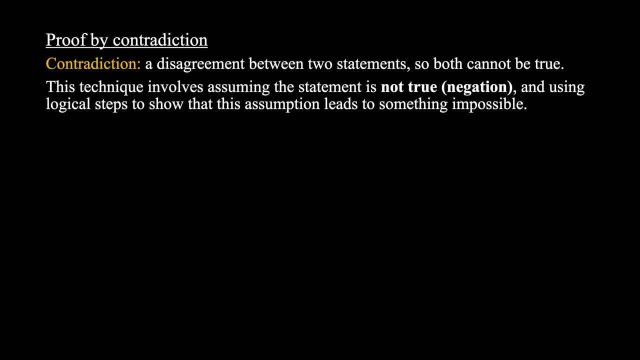 the statement is not true. This is called the negation of that statement, and using logical steps to show this assumption leads to something impossible. Now, writing negations can be tricky, So I'm going to look at an example specifically on a negation before we look at an example of proof by contradiction. So this example says: 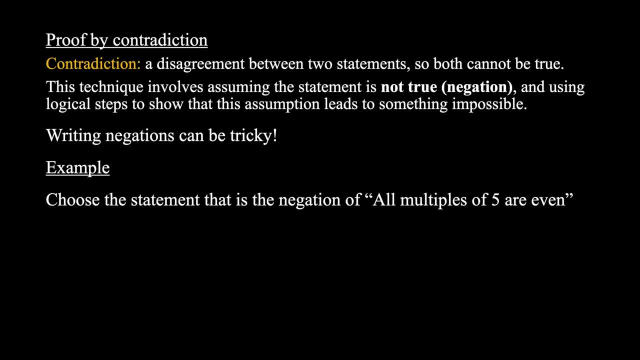 choose the statement that is the negation of. all multiples of five are even. So we're going to have three options: All multiples of five are odd, At least one multiple of five is odd, and no multiples of five are even. which of these is the negation of this statement? 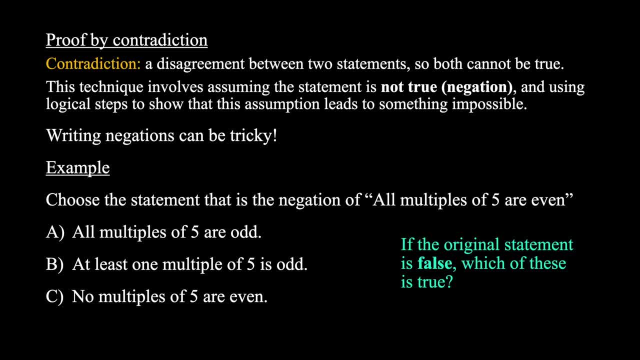 Another way to think about this is to ask the question: if the original statement is false, which of these statements is true? So, if this statement all multiples of five are even is false, would that mean that all multiples of five are odd? Would we have enough information to say, if this was false, that all multiples of five are odd? 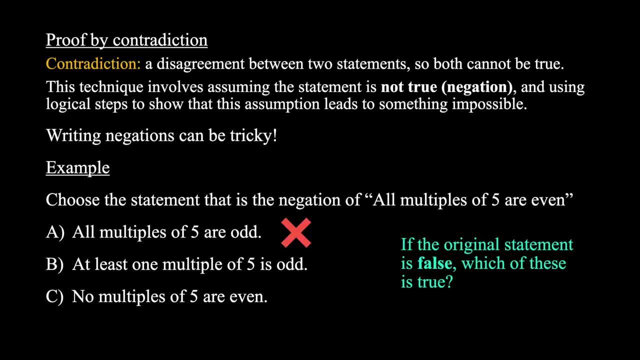 No, we wouldn't. So this is not the negation of that statement. What about C? Would we be able to say that no multiples of five are, even if this is false? No, The only thing we could say if this statement is false is that at least one multiple of five is odd, because that would mean 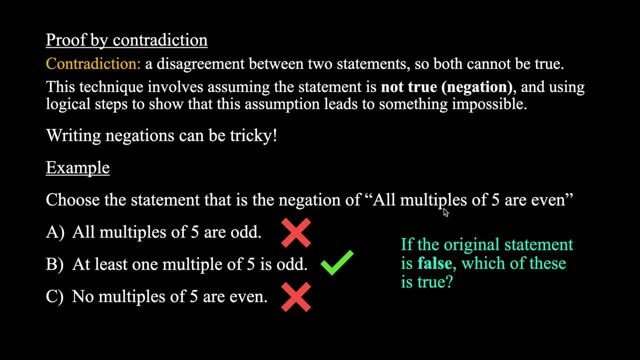 then that this is wrong, that not all multiples of five are even So B there is the negation of this statement. Okay, maybe you agree with me now that this looks like it could be tricky sometimes, but I hope that example helps it to make sense. Let's look at an example of proof by: 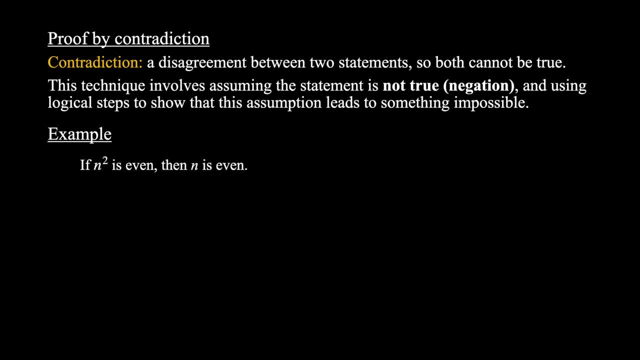 contradiction. Then this statement says: if n squared is even, then n is even. So try to think of the negation of this statement. In other words, if this statement was false, what would that mean? Well, we would still have that n squared is even, but what would it mean about n? We're trying to figure out something. 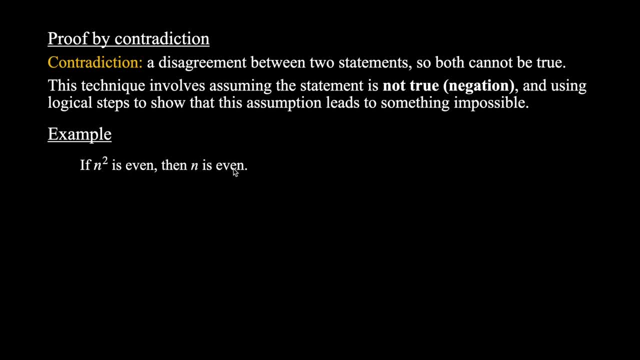 about n. If n is not even, what would it be? Well, it must be odd, right? If n is not even, then it must be odd. So the negation of this statement is that n squared is even and n is odd. So this is what we. 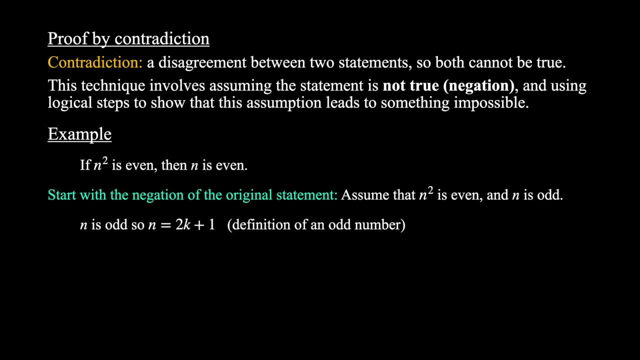 start with We assume this is true and then we can say that if n is odd, n equals 2k plus 1.. This is the definition of an odd number, One more than a multiple of two. Then we can square n, So n. 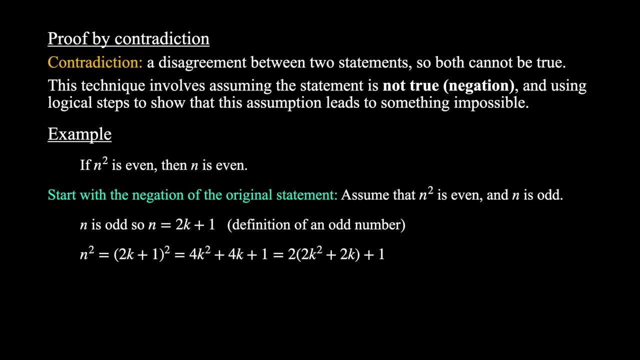 squared is 2k plus 1 squared, which is 4k squared plus 4k plus 1, and we can factorize the two out of the first two terms. So this will be 2 times 2k squared plus 2k plus 1, and clearly this is an. 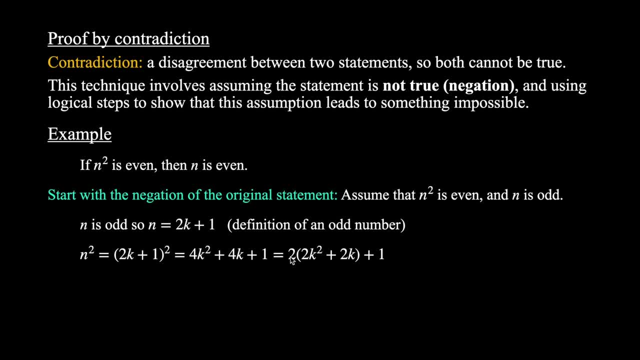 odd number. This is one more than a multiple of two. So by definition this is an odd number. So this is the general process of proof: by contradiction, You start with the statement that is the negation of your original statement. Assume that's true, Follow some logical steps and then. 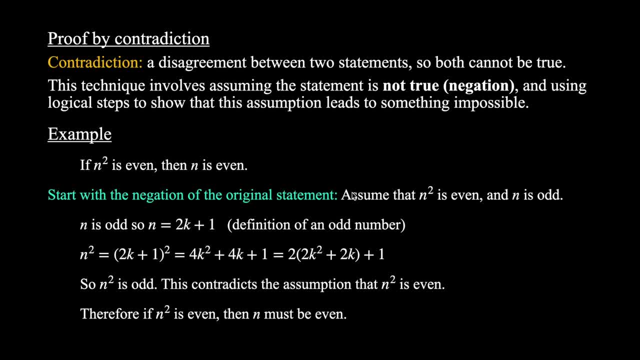 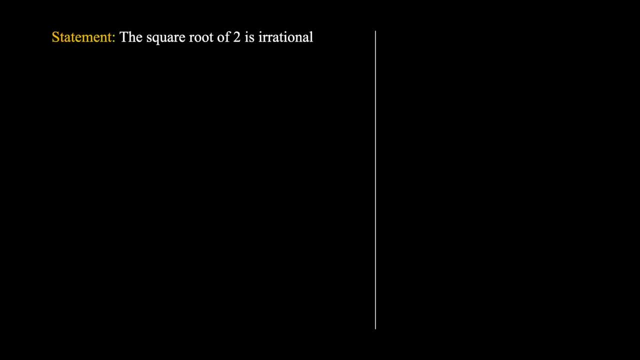 when you get to a contradiction that proves that this statement is false, and the negation of that must be true. Let's look at another example Proof by contradiction. This one is the statement that the square root of 2 is irrational. I'll give 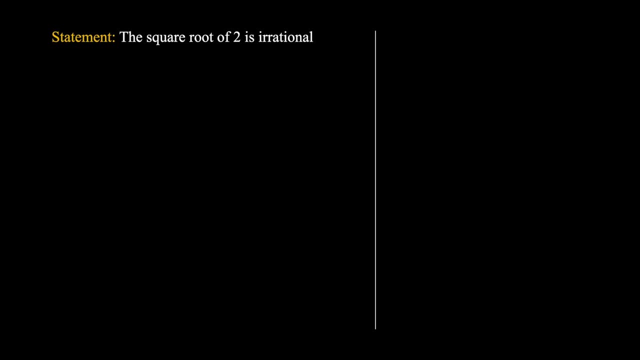 you a moment to think about what would be the negation of this statement. If the square root of 2 is not irrational, what would it be? It must be rational. So we start with the negation. We assume that the square root of 2 is a rational number and we can assume that it's, in simplest, 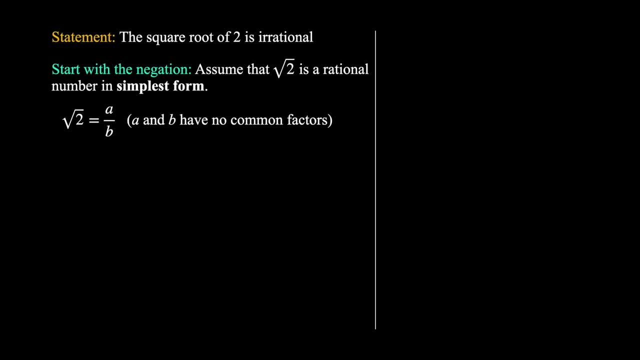 form. So we can say the square root of 2 equals a over b, where a and b have no common factors. This is the definition of a rational number. We can write it as a fraction and we can assume it's in simplest form, because we could just cancel any common 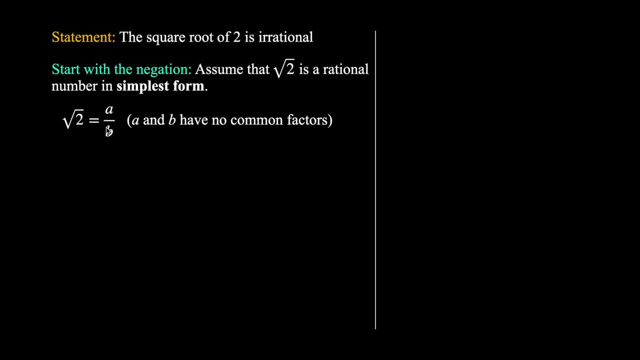 factors. So we've fully simplified this rational number into a over b. So we're assuming this is true. So we can square both sides and we would get a squared on b squared equal to 2, and then multiply both sides by b squared So we get a squared equal to 2, b squared. and because a squared 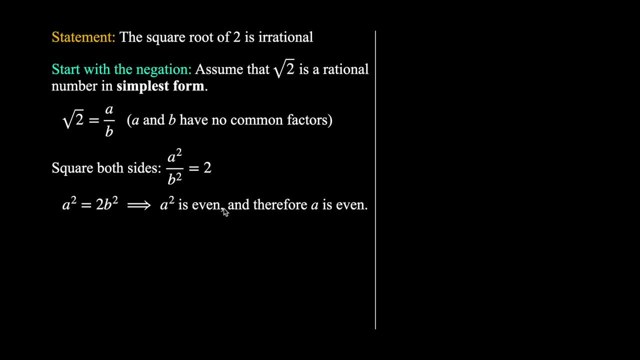 is a multiple of 2. that means a squared must be even and, as we just proved, that means that a must be even. So now let's let a equal 2c, So some even number which is a multiple of 2.. This is the definition. 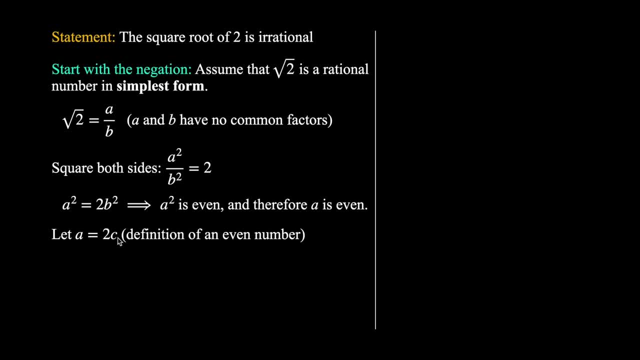 of an even number, and then let's substitute 2c into this equation here. So we're substituting 2c for a. Therefore we get 2c squared equal to 2b squared. and if we square that 2c squared, we get 2b squared equal to 4c squared. So squaring that term there, and then we can divide. 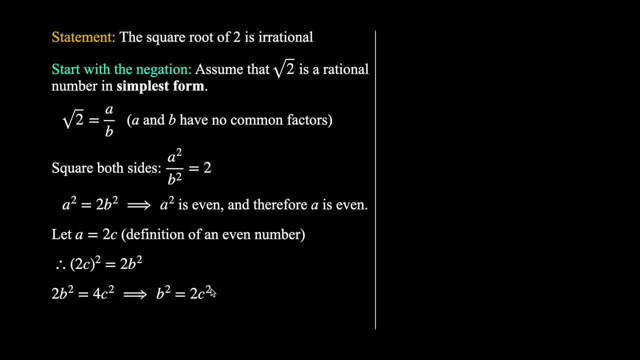 both sides by 2 and we get b squared equal to 2c squared. What does this mean? That means that b squared is even and so b is even. This is a contradiction because, remember, we assumed this was a fraction in simplest form. So this is a contradiction, as we assumed a and b had no common. 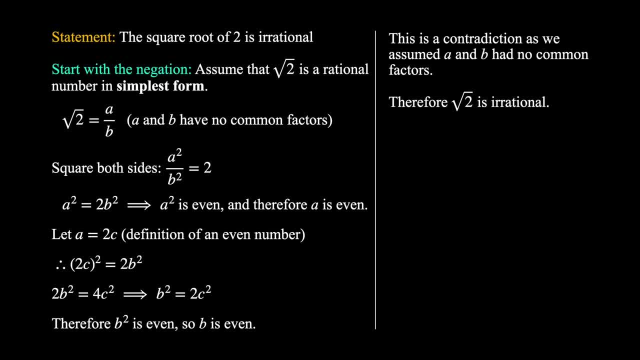 factors, and so then we can finish the proof by saying: therefore, the square root of 2 is irrational. Now, if you're as stubborn as I was when I first saw proofs like this, you might say: well, what if this fraction just was not in simplest form, And maybe you accept that a and b are even. 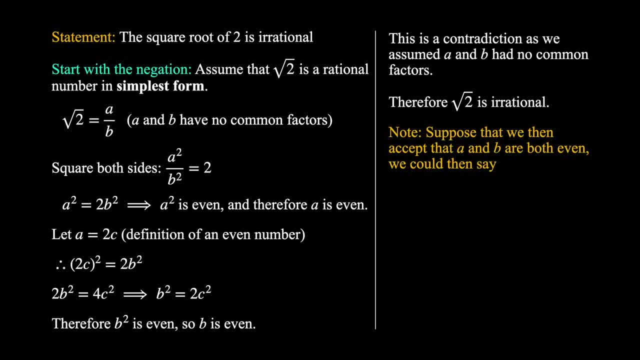 and we could keep going. So let's consider that case. So suppose we then accept that a and b are both even. We could then say that the square root of 2 equals e on f. So we've divided a and b by 2. 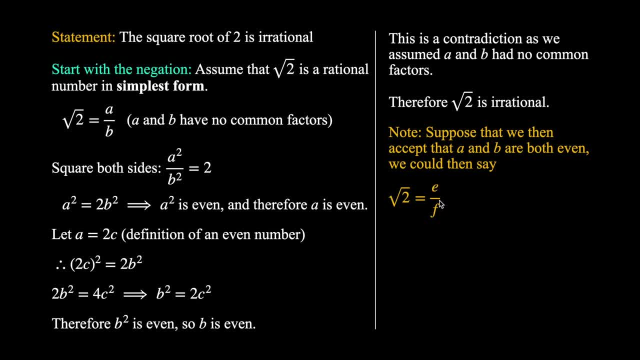 and we've got a simplified fraction e on f. The problem with this is we could then continue this process, So we could use this same method, and we could use this same method, and we could use this same argument and continue this infinitely many times. This is also a form of contradiction.